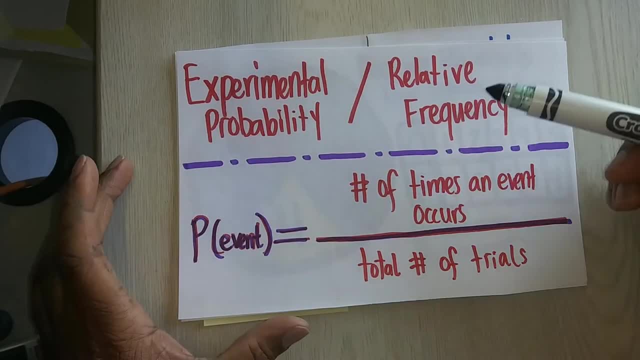 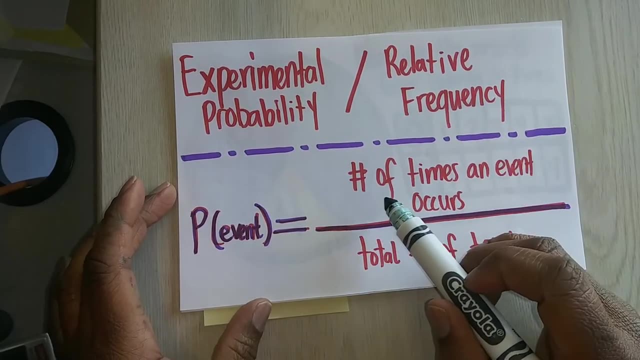 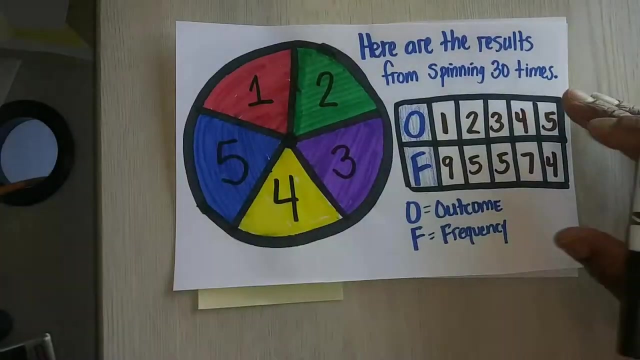 is called experimental probability. Now there is a formula that you can use to determine experimental probability, and what you would do is you will figure out the number of times an event occurred and divide that by the total number of trials. So let's take a look at this example here. 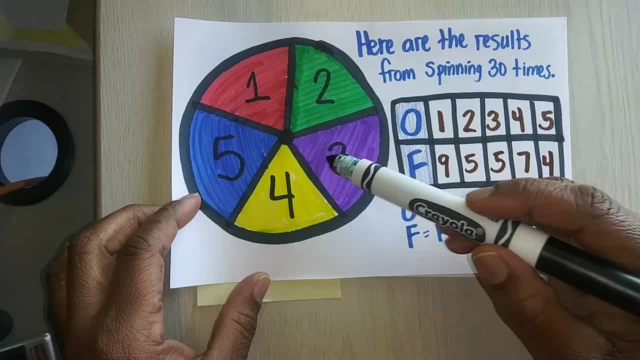 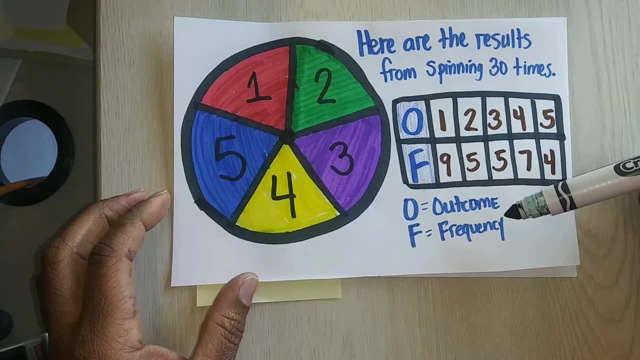 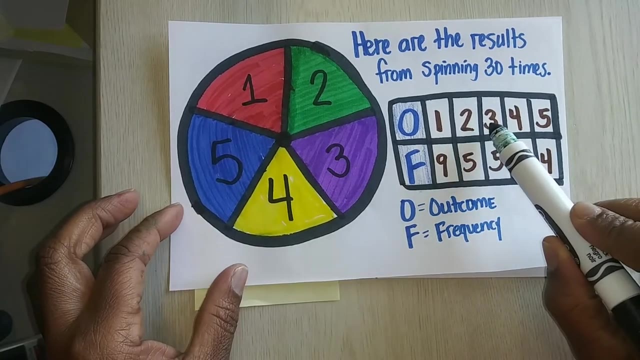 So here I have a spinner with five sections with different colors And with that I have these results after 30 spins. And after 30 spins, the outcomes: either it could land on the number one, the number two, the number three, the number four, or it could land 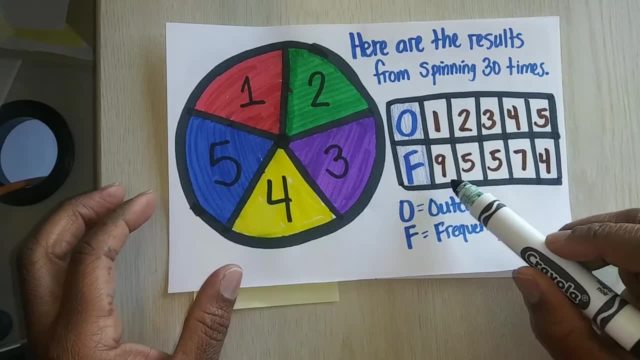 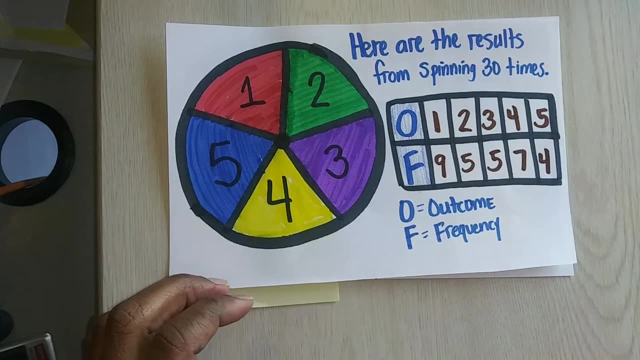 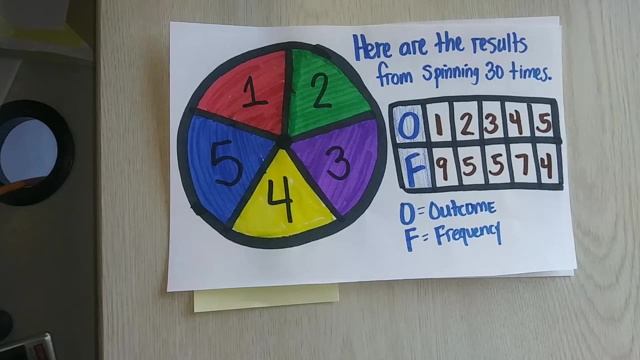 on the number five, and the f represents the frequency on how often it occurred. So it landed on the number one nine times when I took my spinner right, and then it also landed on the number two five times, And then it landed on the three five times, and then it landed on the four seven times. 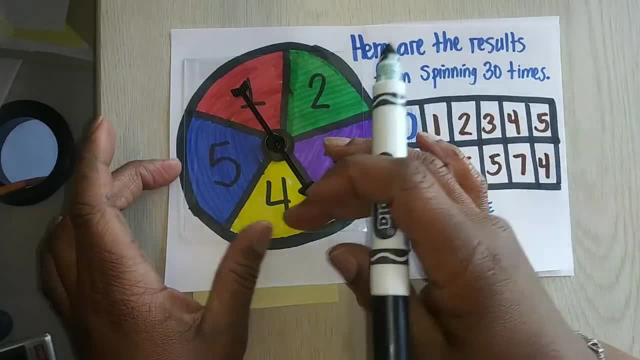 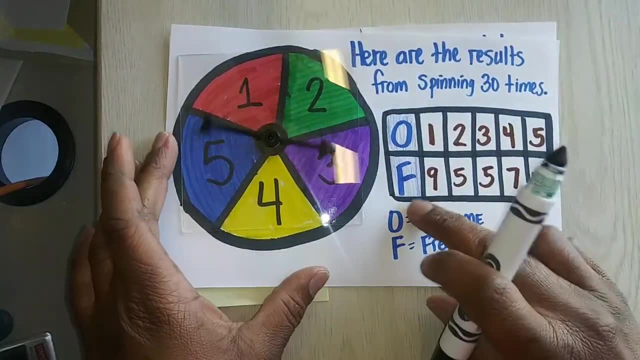 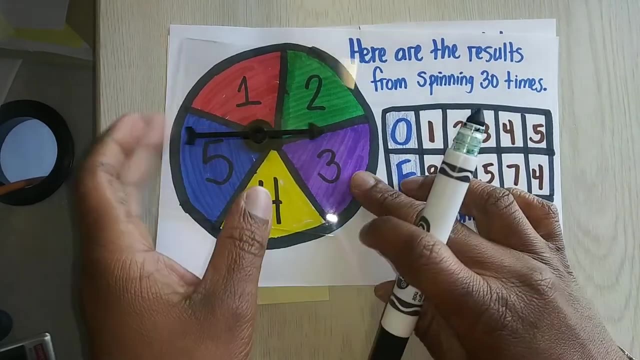 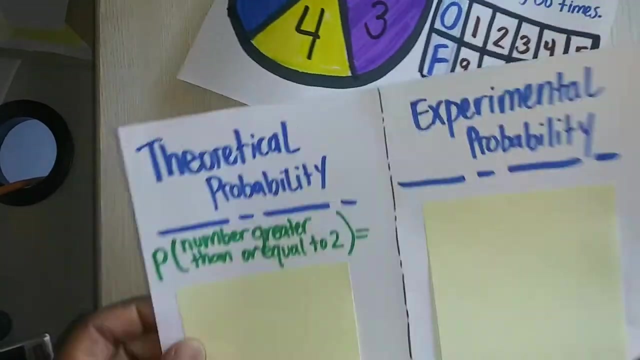 and the number five four times. So basically, after I put my spinner here and I spin and I spent it, the probability, or the frequency, is how I got that every time I actually spent the spinner. All right, so using that information, we are going to actually take a look at this here. 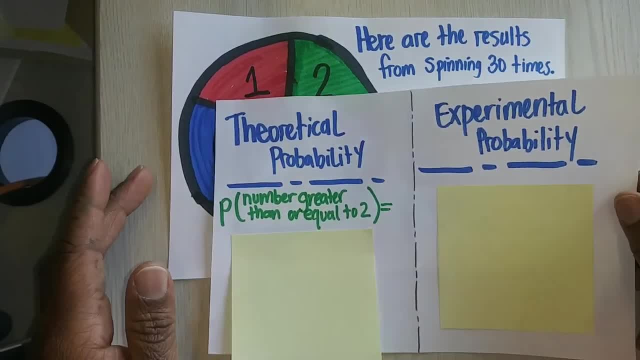 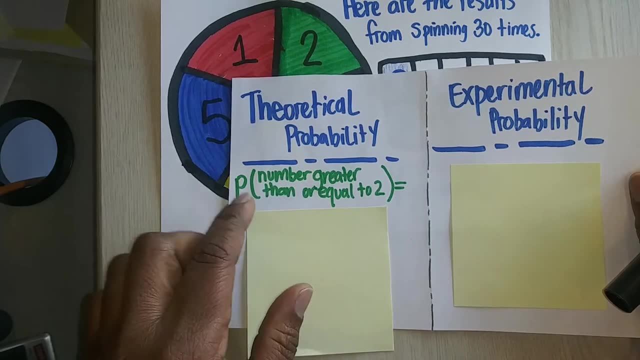 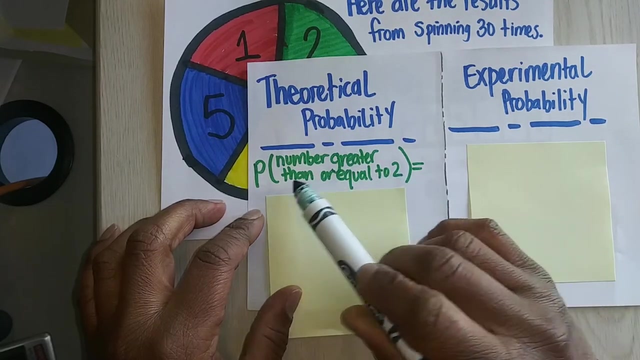 So I want to know the theoretical probability and the experimental probability. So with the theoretical probability, that's what the math tell us should occur. So if I'm looking for any number that's greater than or equal to two- the probability- well, let's see how. 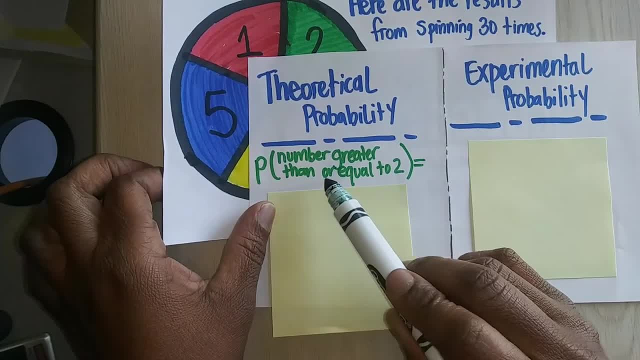 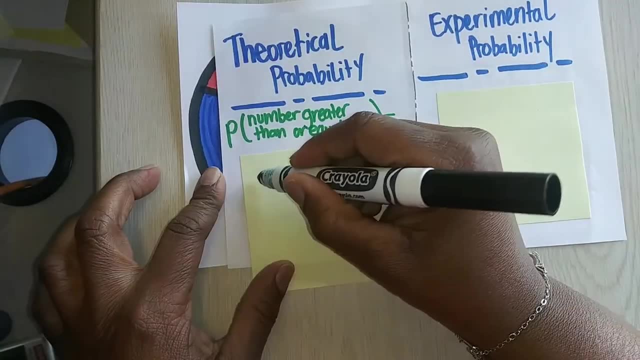 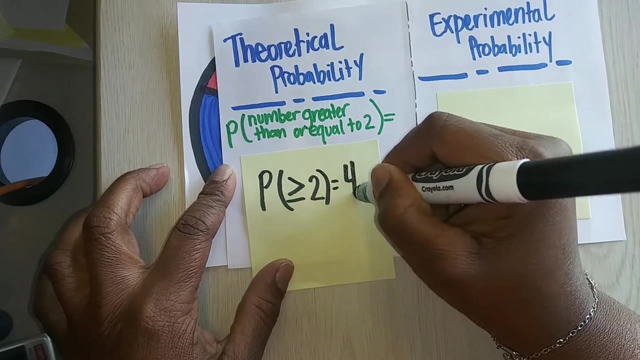 many numbers we have that is not only greater than, but is also equal to the number two, So that will be one, two, three, four, And in this case The probability of getting a number that's equal to or greater than two would be four out of five possible outcomes. right, because it's labeled one through five. 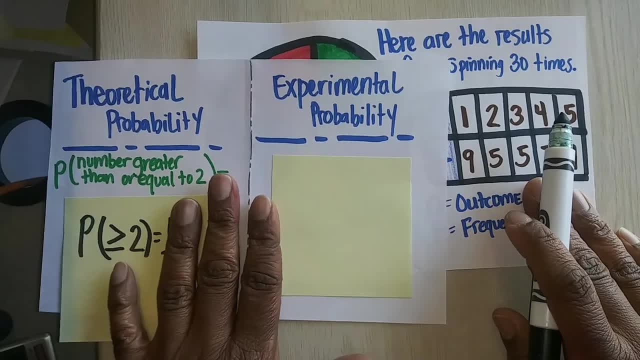 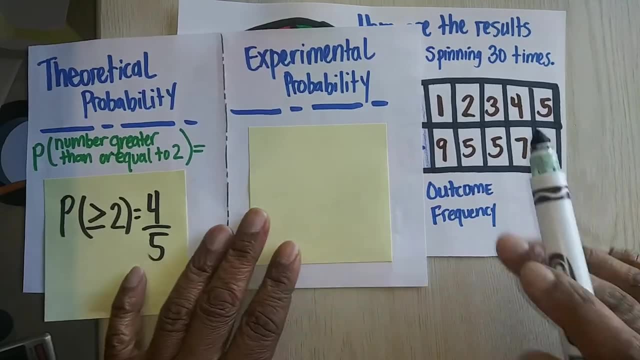 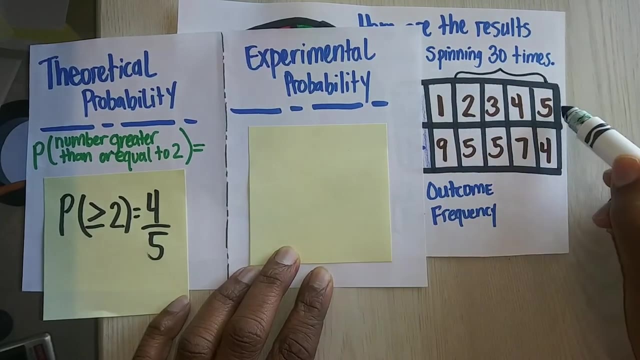 Now the experimental is what actually happened And in this case the number of trials or the outcome that was greater than or equal to two is right here. So it could be anything from here To here, Equal to or greater than two. So five plus five is ten. Ten plus seven is seventeen.